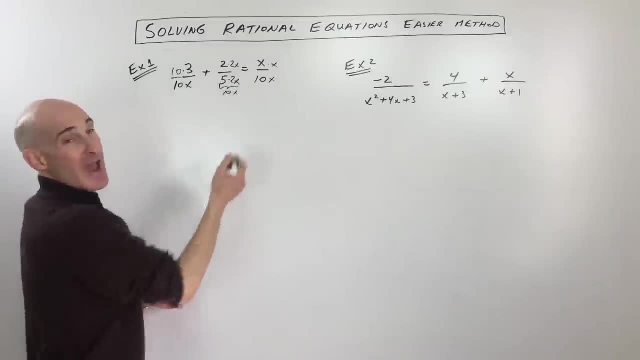 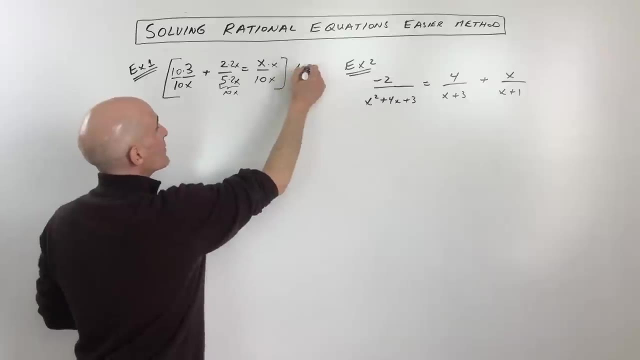 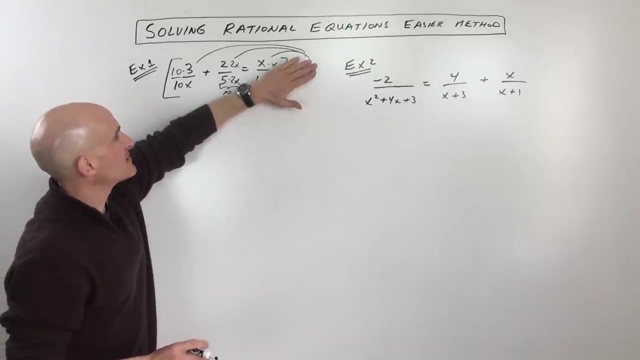 so now you can see that all the denominators are 10x. So now what I would do is I would say: all right, I'm going to multiply everything by this denominator, 10x. So when you do that, when you distribute it, okay, what happens is when you multiply the 10x and the 10x, those are going to 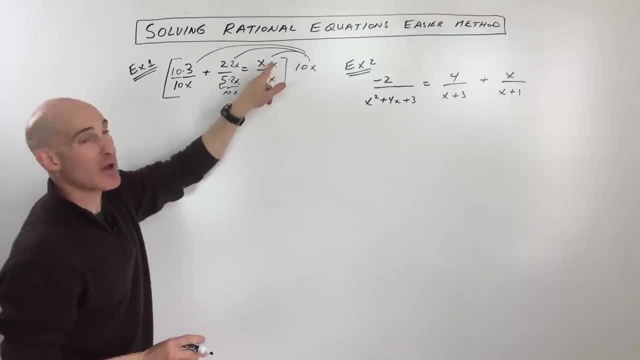 cancel. So what it does is it clears the denominators. You don't want to actually multiply the numerators by 10x, You just want to realize that, since these all have the same denominator, if you were to multiply through by that common denominator, you're just going to be. 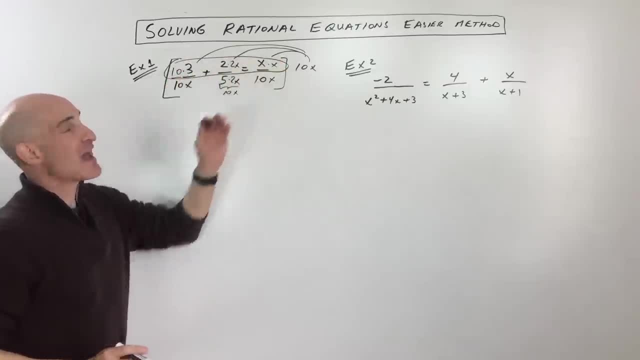 left with the numerators. So are you with me so far? So we're just going to have those numerators. all the denominators are the same. You can ignore those, because they're going to cancel out if you multiply by that common denominator, 10x. So what we have here now is 30 plus 4x equals x squared. 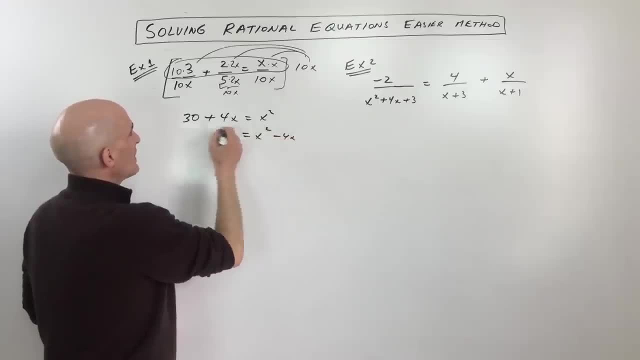 I'm just going to get everything on one side by subtracting 4x and subtracting 30.. Set that equal to zero. Now what you can do is you can try to factor it, or you could do the quadratic formula, or you could complete the square- Any of those techniques- so that you can find out what x is. 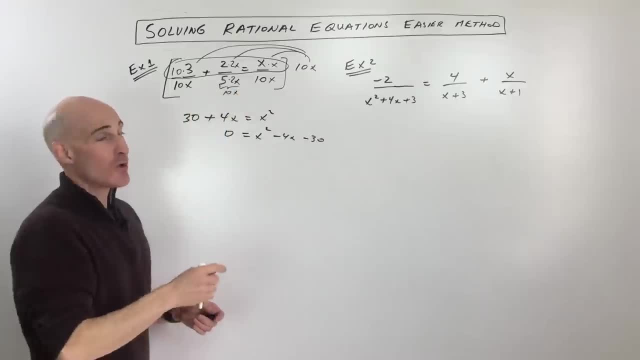 but the main thing is, you want to make sure that the denominator is not zero. So in this case, if x came out to zero when we solve this, then that means that it's no solution, That's a false answer or an extraneous solution. So this would involve- I would probably do the 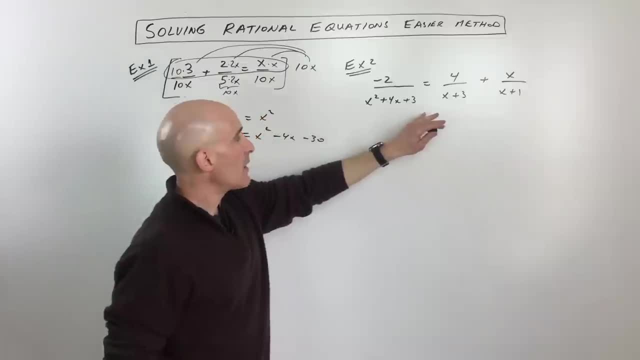 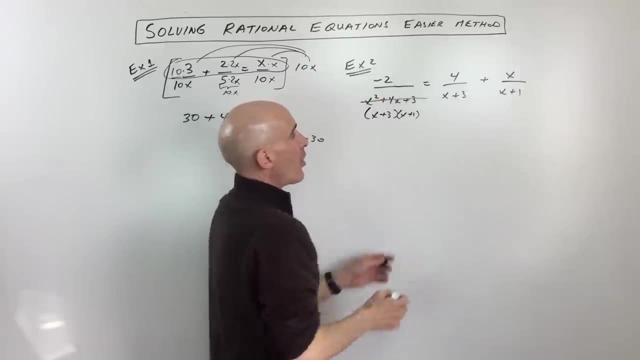 quadratic formula. Now let's go over to example number two, Now this one. what I recommend doing first is factoring the denominator, Okay, all the denominators, So you can see what they're all composed of or what they're made up of. right, So you can see: this one has an x plus 3, but it's. 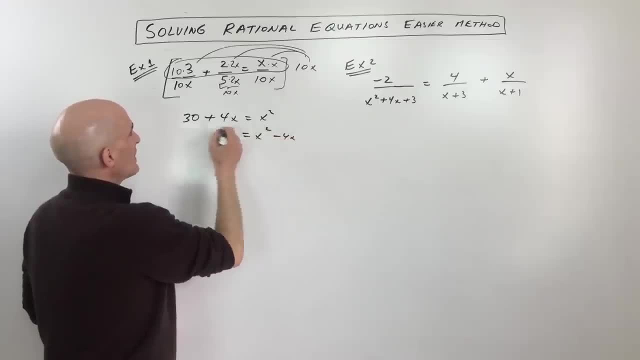 I'm just going to get everything on one side by subtracting 4x and subtracting 30.. Set that equal to zero. Now what you can do is you can try to factor it, or you could do the quadratic formula, or you could complete the square- Any of those techniques- so that you can find out what x is. 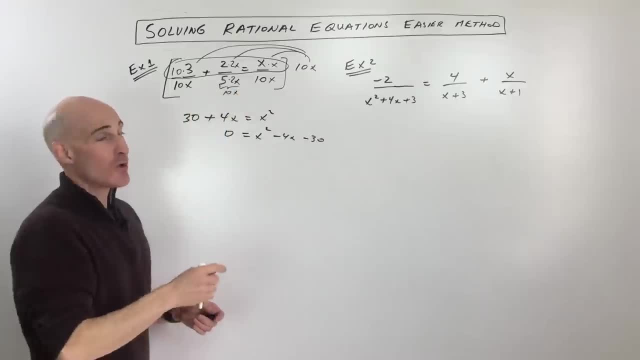 but the main thing is, you want to make sure that the denominator is not zero. So in this case, if x came out to zero when we solve this, then that means that it's no solution, That's a false answer or an extraneous solution. So this would involve- I would probably do the 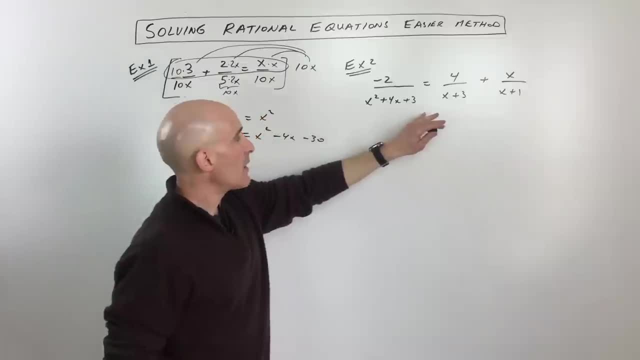 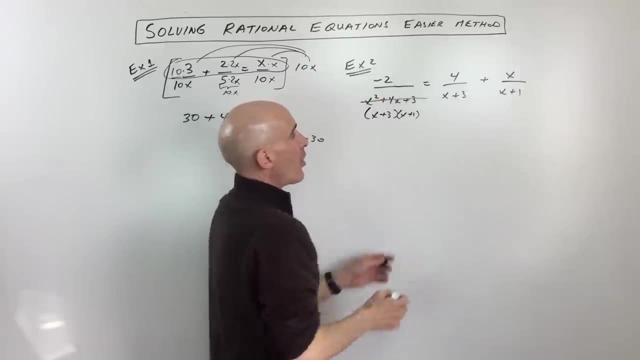 quadratic formula. Now let's go over to example number two, Now this one. what I recommend doing first is factoring the denominator, Okay, all the denominators, So you can see what they're all composed of or what they're made up of. right, So you can see: this one has an x plus 3, but it's. 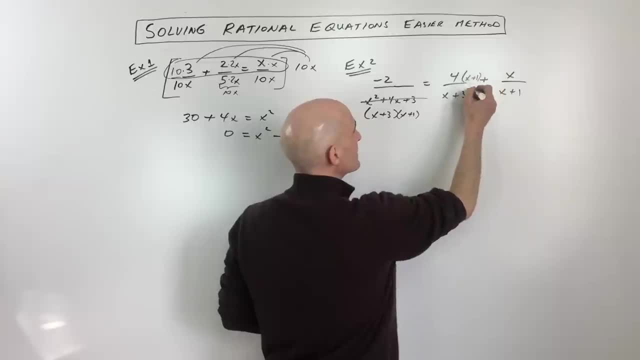 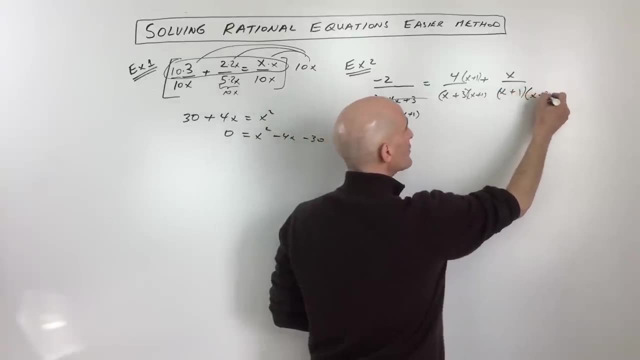 missing an x plus 1.. So what we're going to do is we're going to multiply by what it's missing, so that it'll have the same denominator. Okay, this one has an x plus 1, but it doesn't have an x plus 3.. See, our goal is to get all the denominators to be the same. Okay, so whatever. 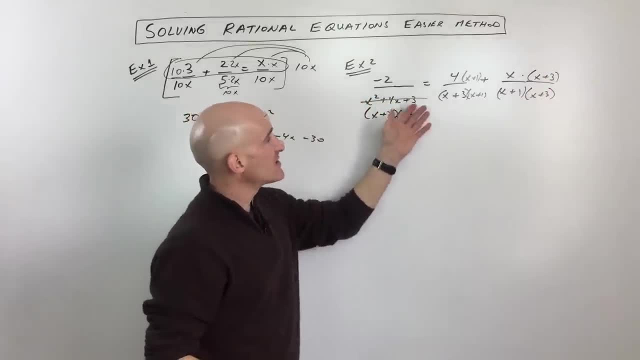 it's missing. multiply the top and bottom by that quantity. Now you can see. okay, they all have the same denominator. So what you can do is you can ignore those denominators. Okay, when I say ignore, I don't mean ignore. I just mean that if you were to multiply through by the common denominator, 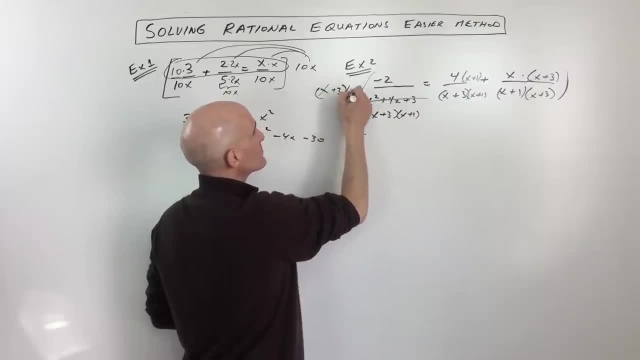 which is x plus 3, x plus 1 right, x plus 3 and x plus 1.. If you were to distribute this to each of these fractions- because this is in the numerator and this is in the denominator- it's going to cancel those out So effectively. what we can do. 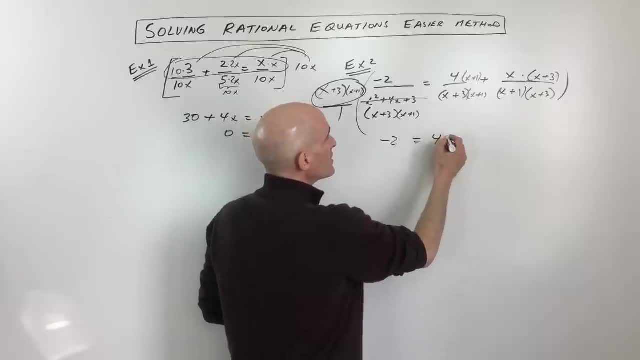 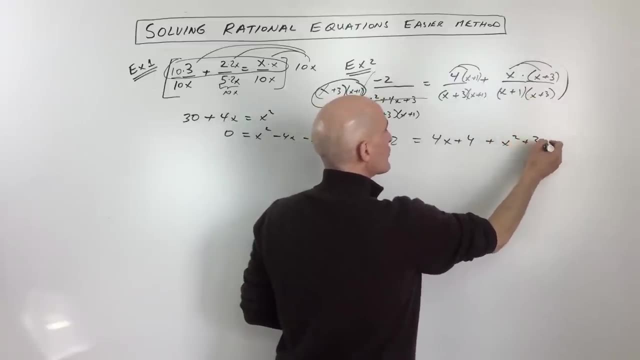 is focus just on the numerators at this point. So what I'm going to do is I'm just going to distribute the 4. Okay, over here I'm going to distribute the x and we're just focusing on those numerators. So now it's a little bit easier to solve because we don't have all those fractions. 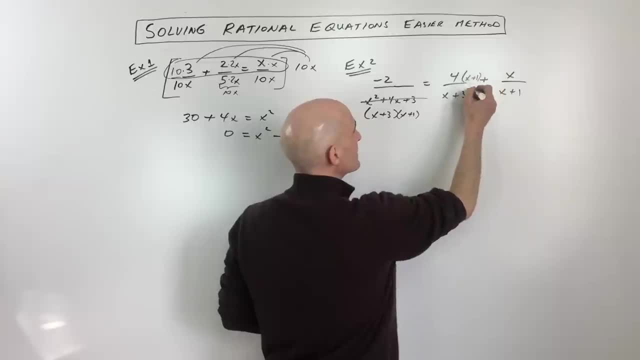 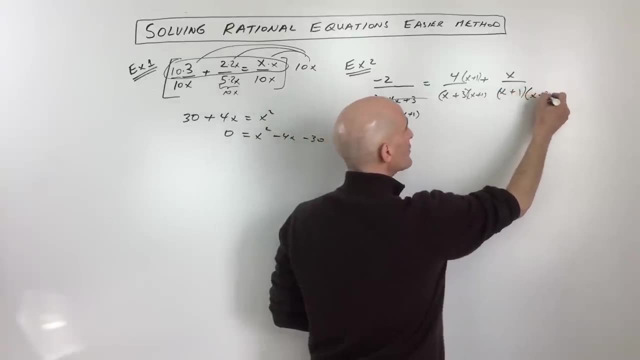 missing an x plus 1.. So what we're going to do is we're going to multiply by what it's missing, so that it'll have the same denominator. Okay, this one has an x plus 1, but it doesn't have an x plus 3.. See, our goal is to get all the denominators to be the same. Okay, so whatever. 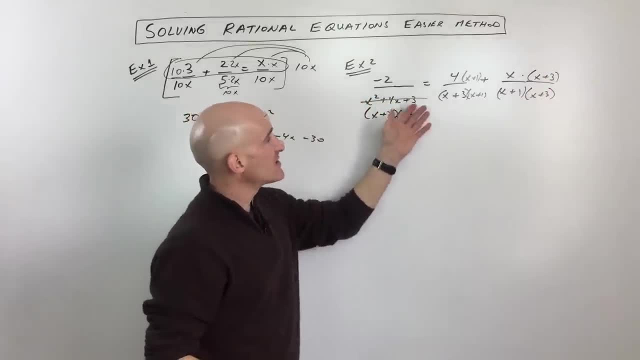 it's missing. multiply the top and bottom by that quantity. Now you can see. okay, they all have the same denominator. So what you can do is you can ignore those denominators. Okay, when I say ignore, I don't mean ignore. I just mean that if you were to multiply through by the common denominator,